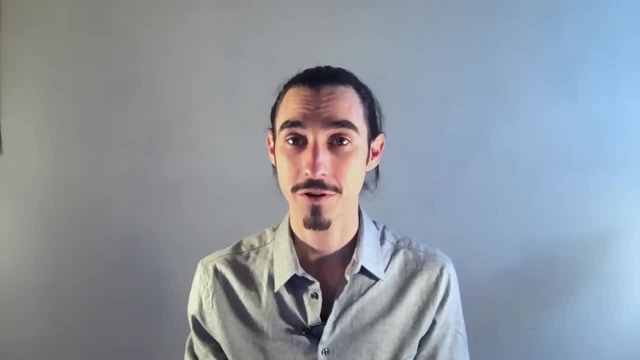 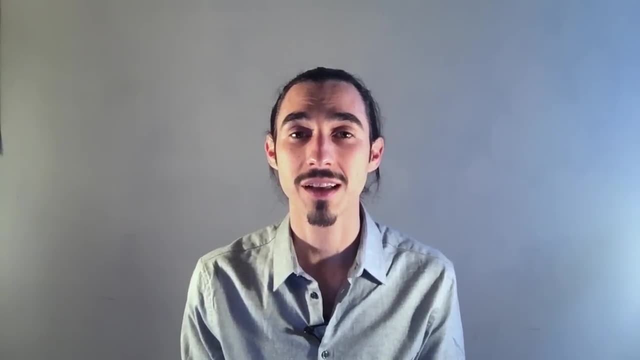 really simple, right? Do it three, four minutes. If you nail it every time you're ready to move on, Let's try another really simple one. We're just going to clap 1,, 3, and 4.. We're going. 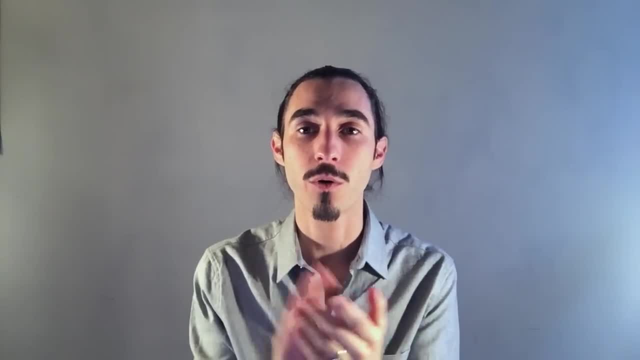 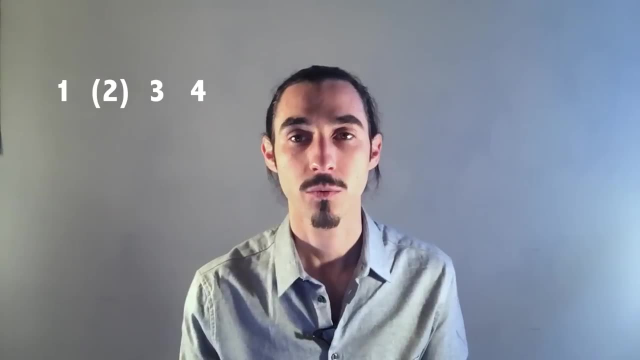 to skip beat two: 1,, 2, 3, 4.. 1,, 2,, 3, 4.. 1. Notice how I make the clap on 1 the loudest. We're at 80 beats per minute. 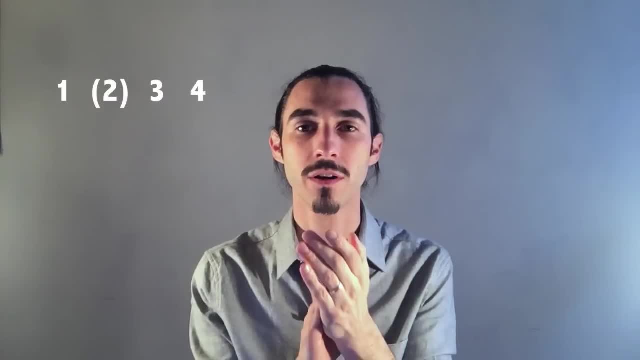 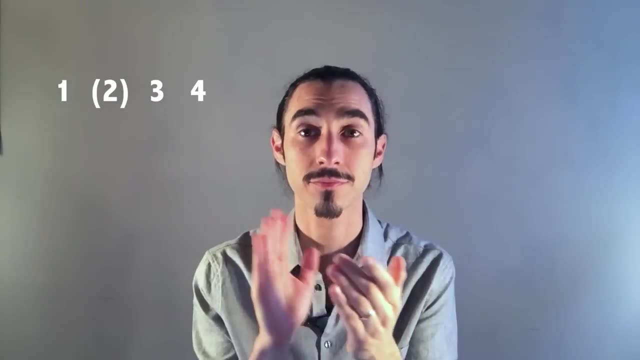 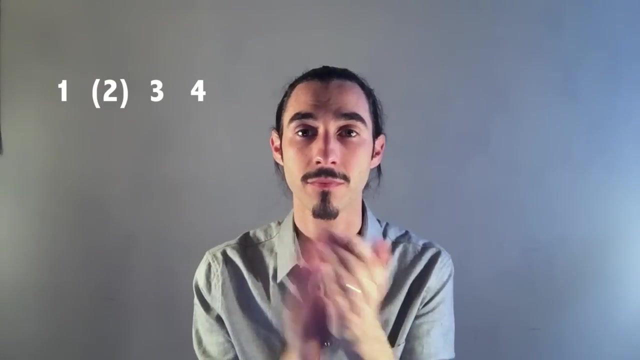 1,, 2,, 3,, 4.. 1,, 2,, 3,, 4.. 1. 1,, 2,, 3,, 4. 1. 1,, 2,, 3,, 4.. 1,, 2,, 3,, 4. 1.. 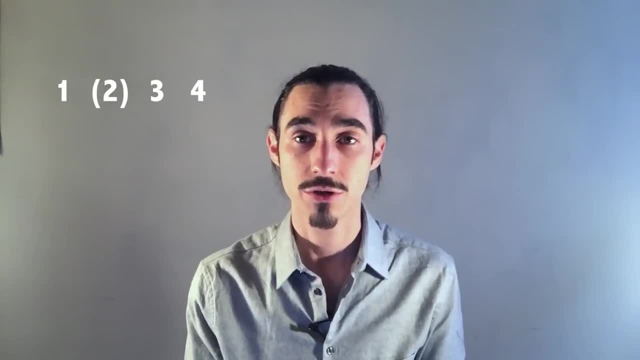 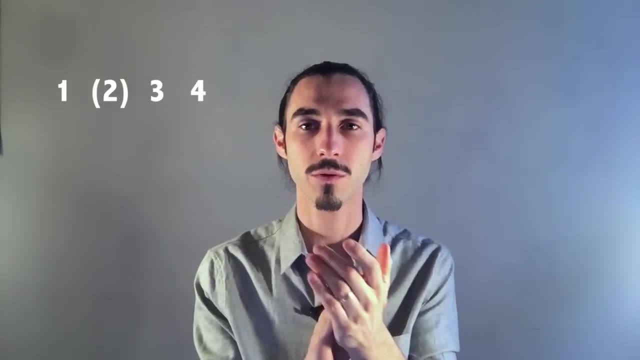 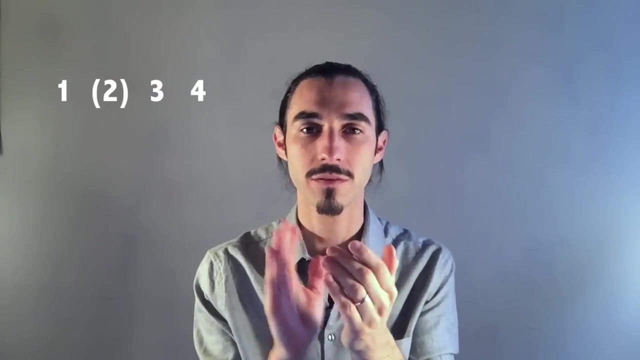 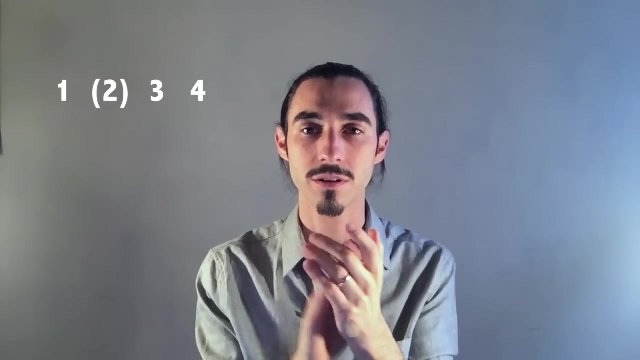 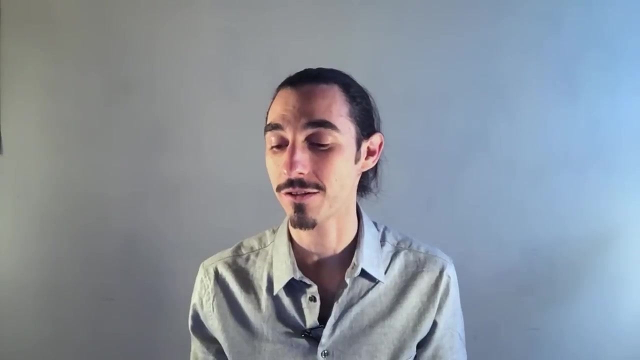 If it seems easy at 80, you could try it a little bit faster. Let's go to 100.. Some of you this seems really simple, right, But I know there's some of you out there that this is already a big challenge. 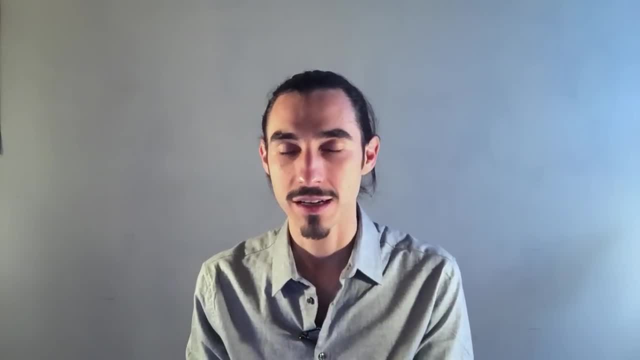 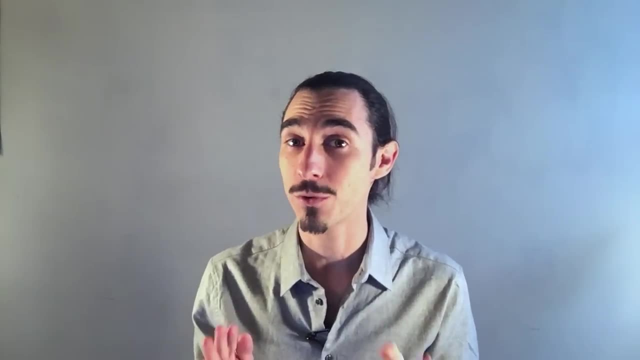 Now what you want to do is start getting into rhythmic subdivision with the metronome. By subdivision, I mean finding the beats between the beats. So what I'm going to do is I'm going to play the metronome again: 80 beats per minute. 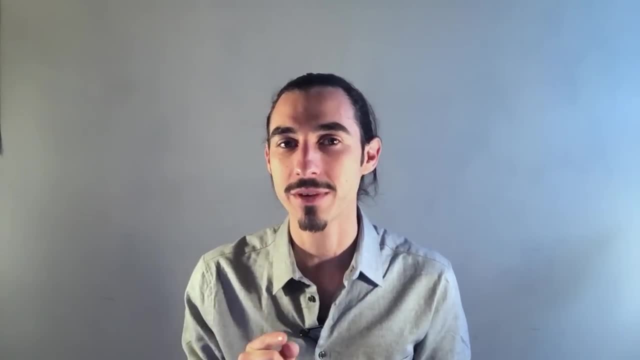 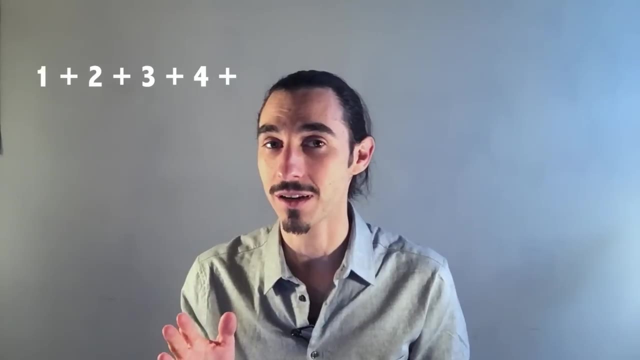 and I'm going to count out loud 1 and 2 and 3 and 4, and These ands, or the beats between the beats, are the subdivisions- Subdivisions that I'm talking about, And once you get a really good feel for the subdivision, you're going to be able to get. 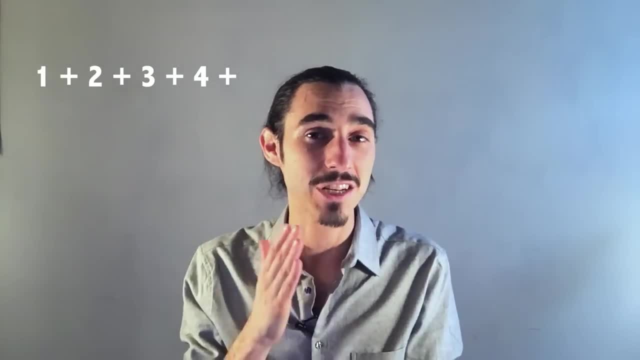 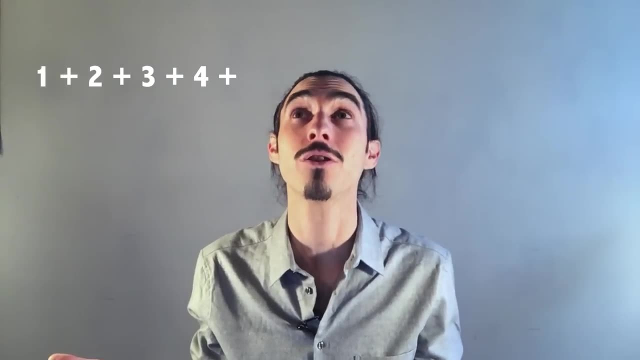 into syncopated rhythms, which means playing rhythms that actually hit on these off beats, And then you get into all the different world music possibilities that are out there, And there are so many. So let's even go down to 60 beats per minute and we're going to start counting the ands. 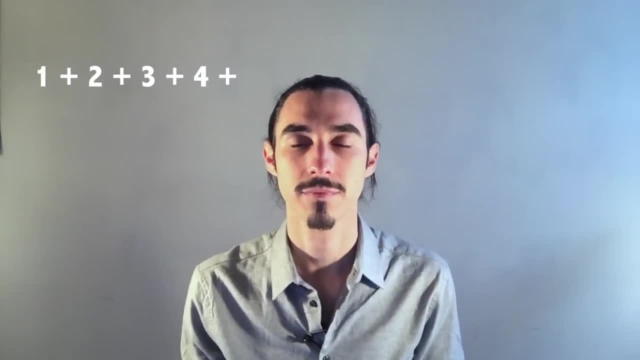 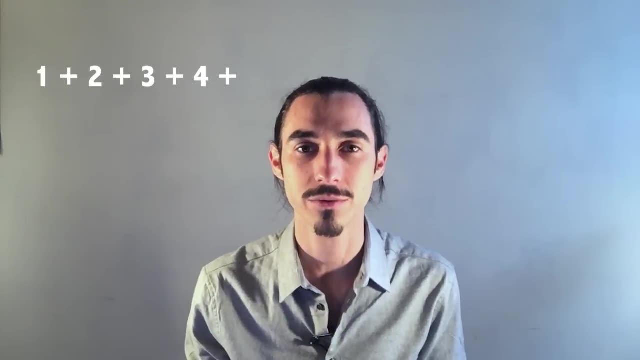 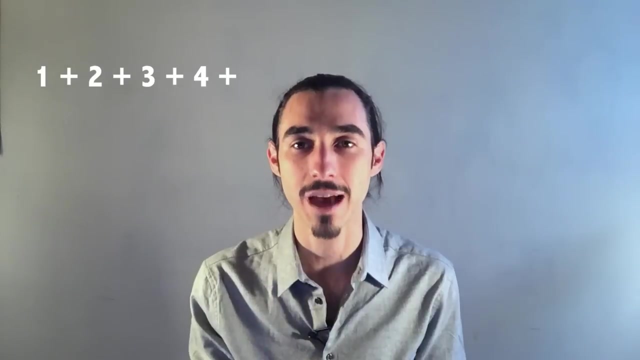 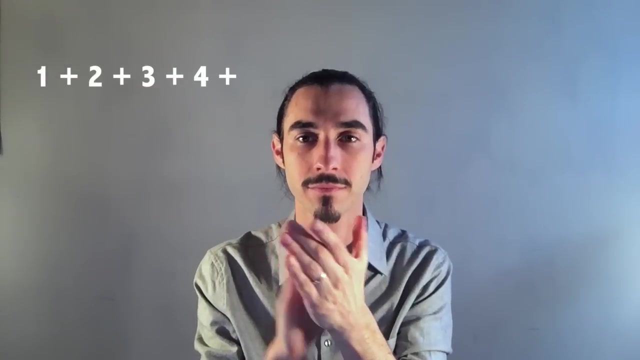 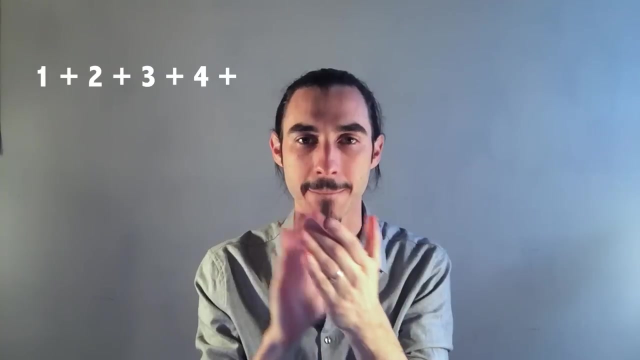 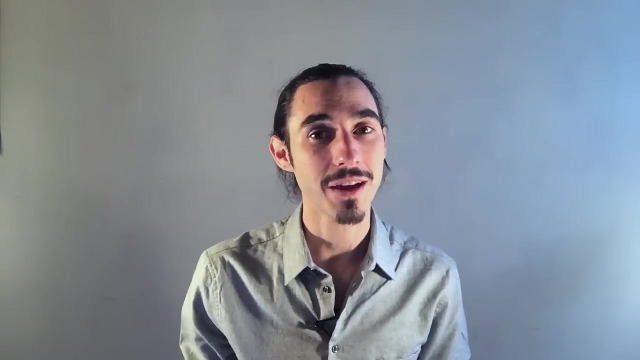 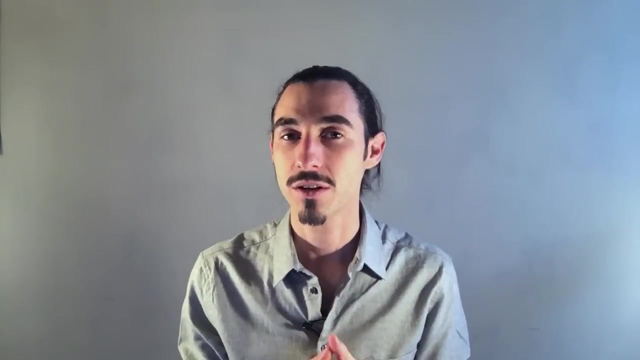 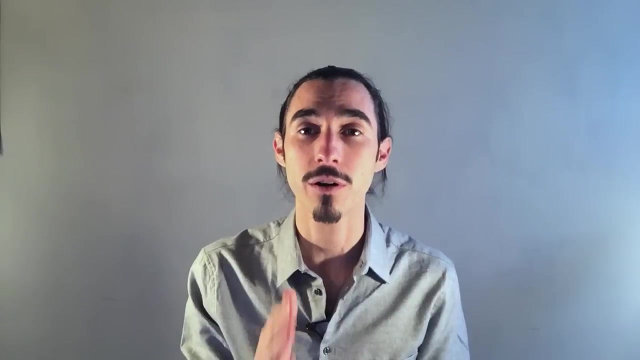 the subdivisions 1 and 2 and 3 and 4 and 1 and 2 and 3 and 4 and 1.. I'm going to start clapping now on the upbeats, the beats between the beats. So now that you can do the upbeats, the ands, and you're also able to clap on the downbeats. 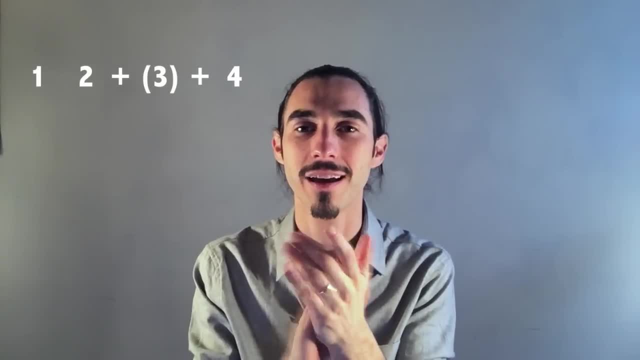 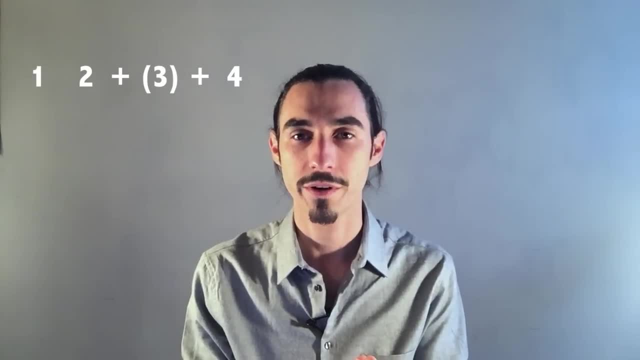 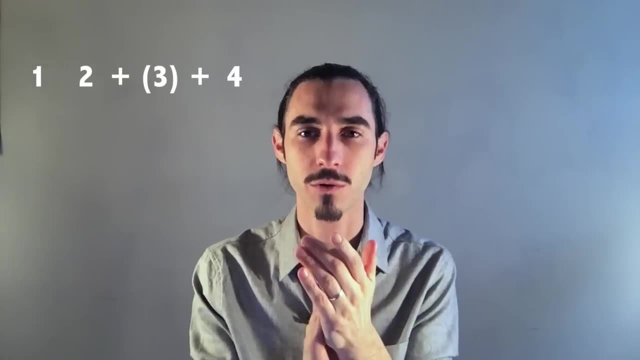 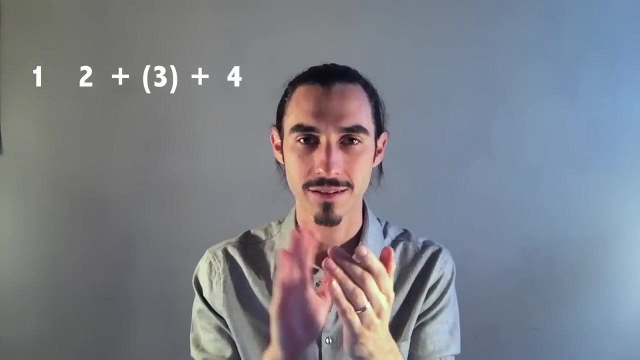 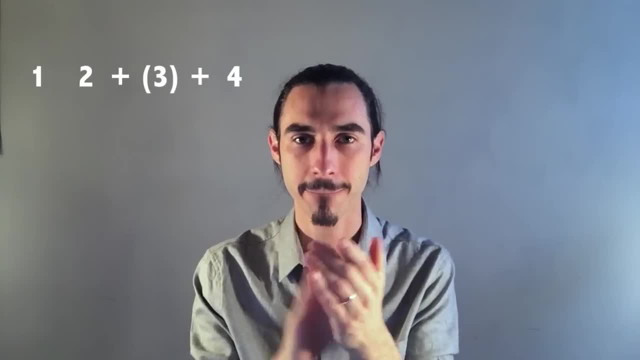 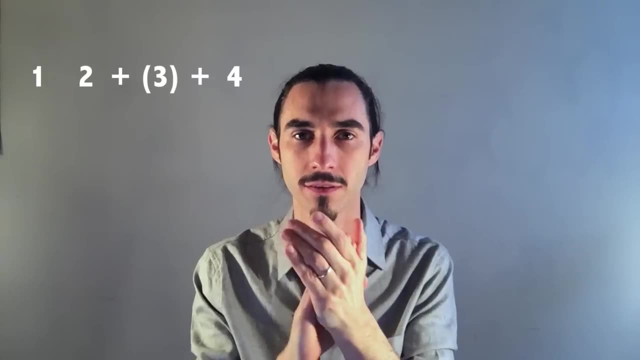 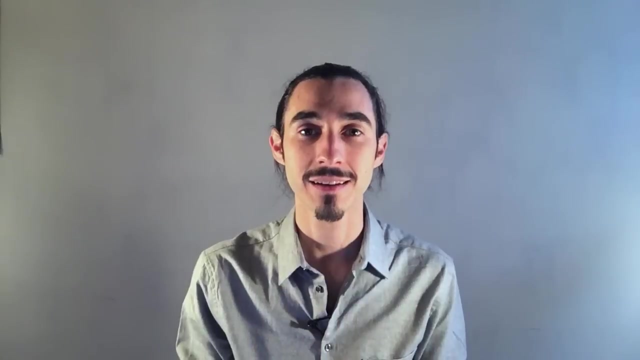 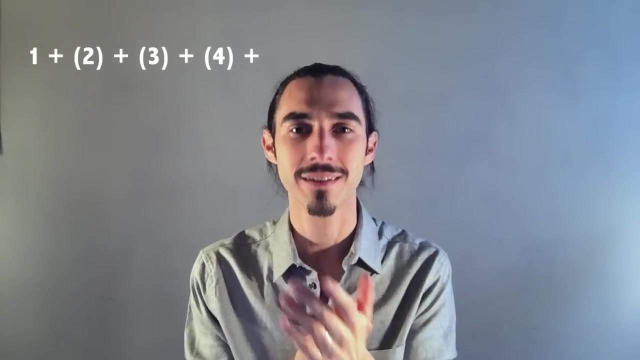 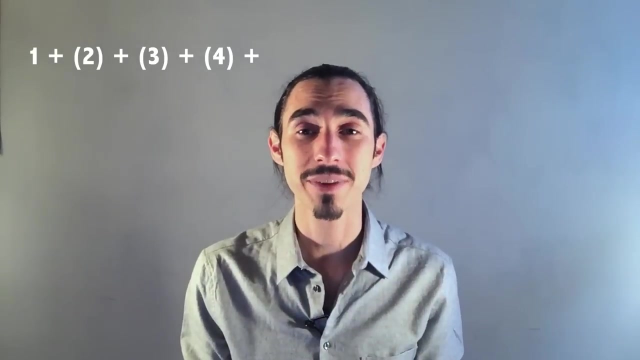 2 and 2 and 4. another one we see a lot in reggae music is one and and and and one and and and and and one, and and and and one, and and and and and. so you're basically playing every upbeat and the only downbeat you're playing is one. so when 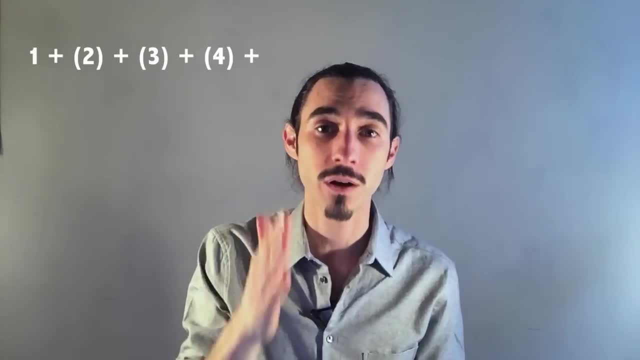 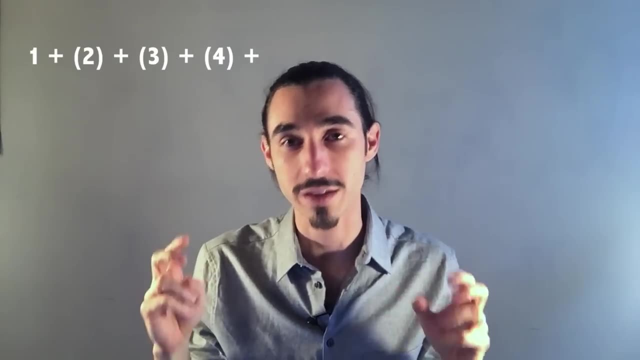 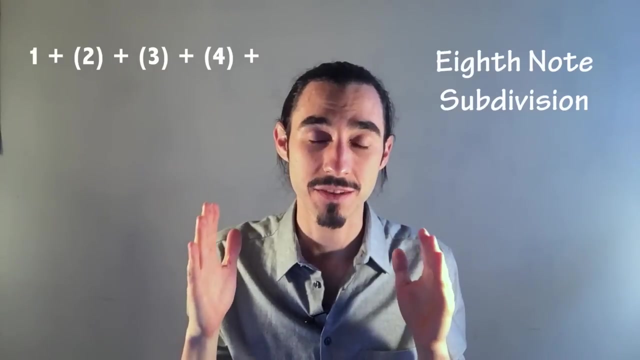 you get to the end of beat four, you're going to go four and one and you have three notes in a row. this technically, in a musical context in like the western music notation, is called eighth note subdivision, because you're dividing the bar into eight sub beats. let's try that one i was singing. 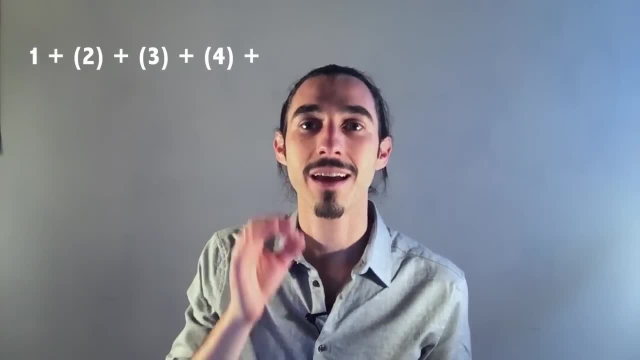 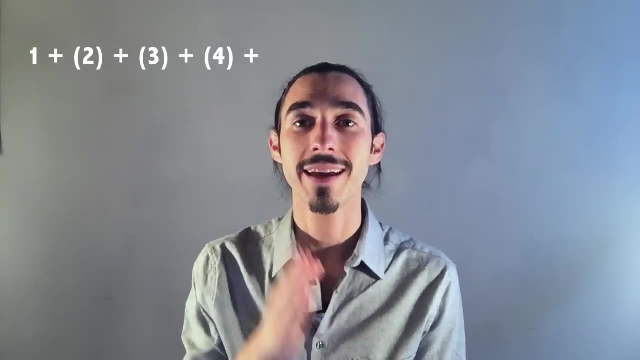 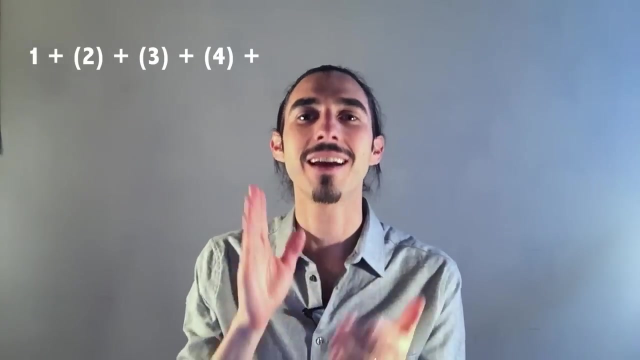 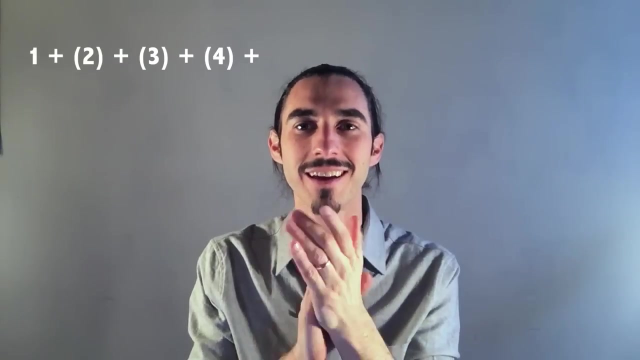 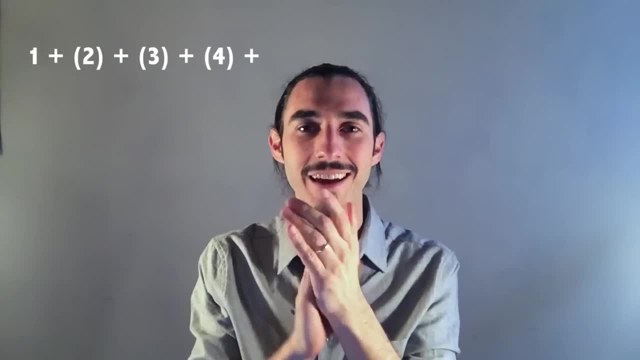 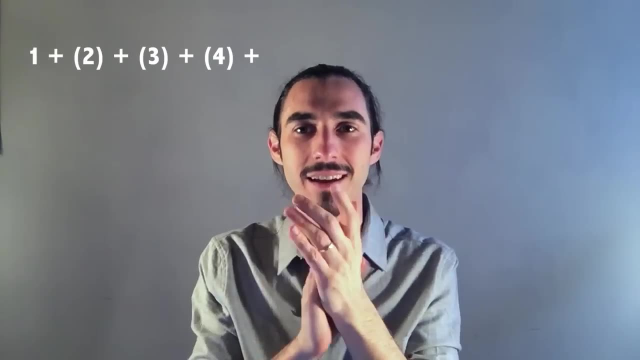 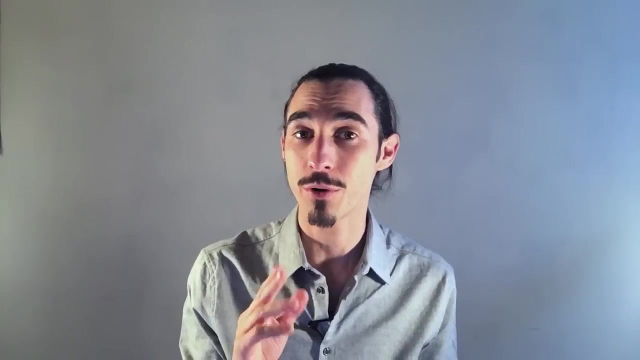 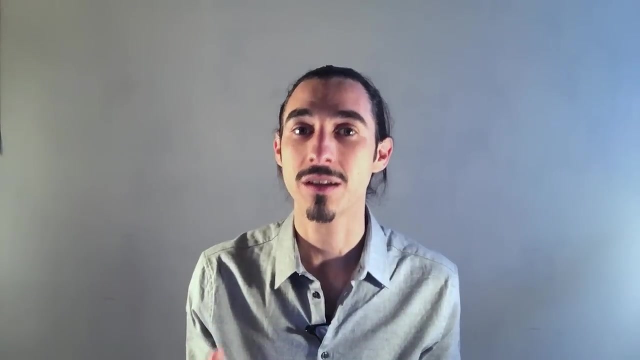 and and and and and one and and and and one and and and and one and and and and. okay, so let's try a world music rhythm that is syncopated, meaning it has both beats on the downbeats and upbeats. that's really popular in all sorts of latin american music, middle eastern music, african music. 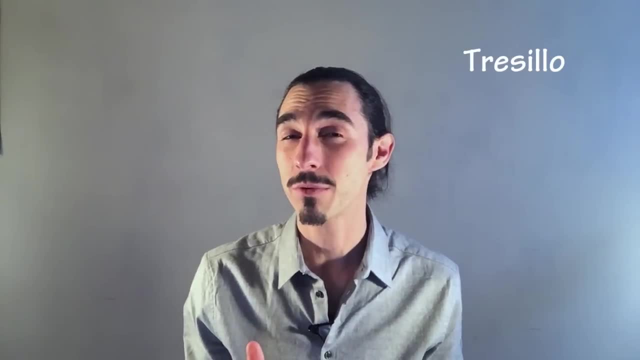 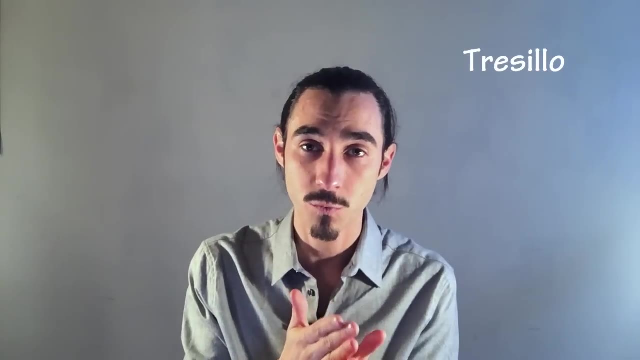 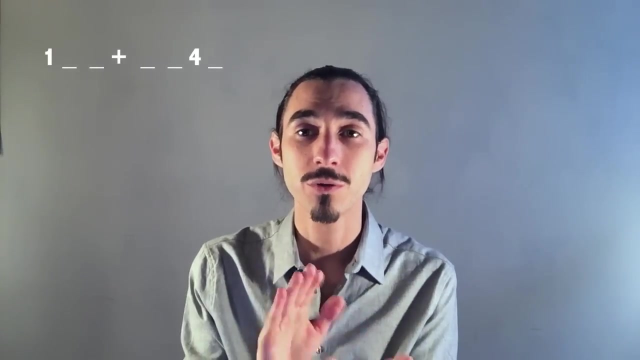 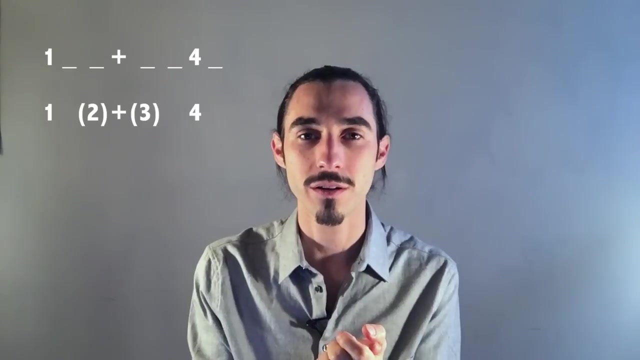 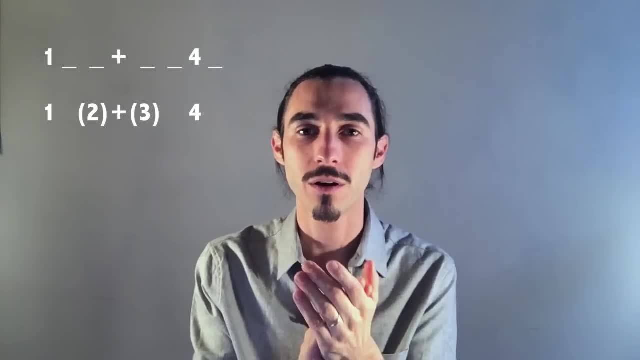 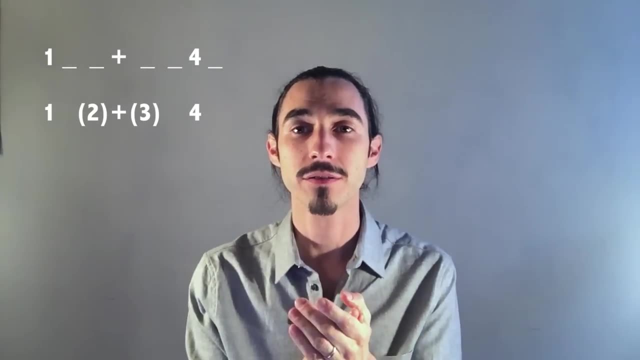 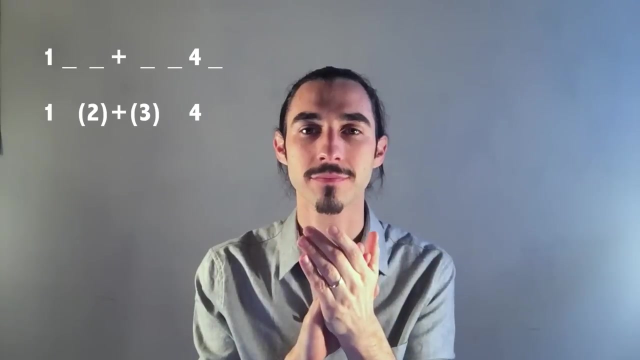 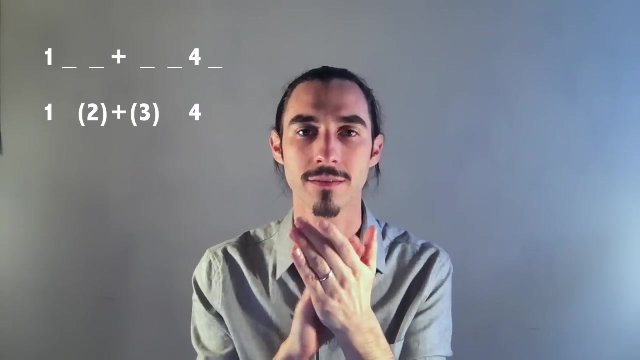 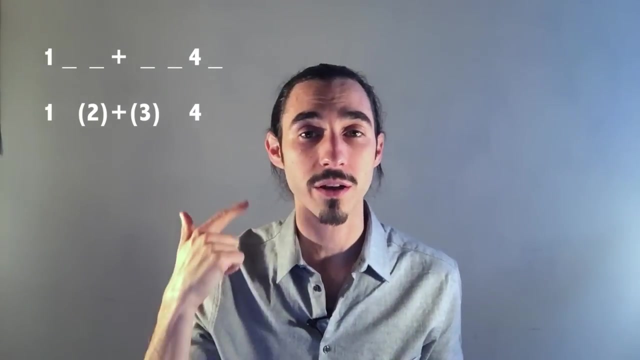 four. one, two and three, four, one, two and three, four. let's try this: 80 beats per minute. one, two and three, four. one, two and three, four helps if, as you're going through it in your head, you go one and two and three and four, and one and two and three and four, and one and two and three and four. 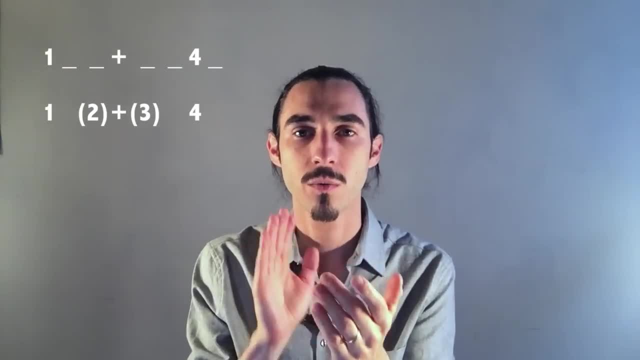 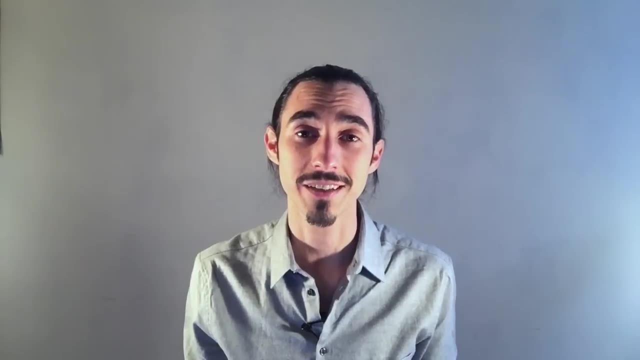 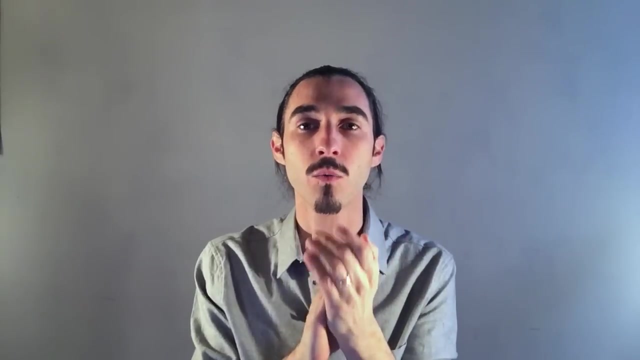 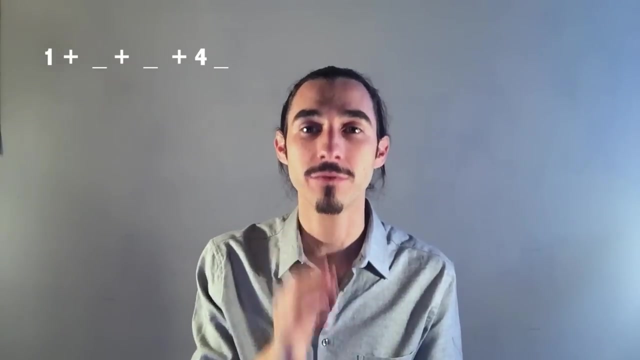 and one and two, three and four and. okay, let's try one that's a little more complicated. let's go one and and and four. one and and and four. one and two and three and four. one and two and three and four. one and two and three and four.